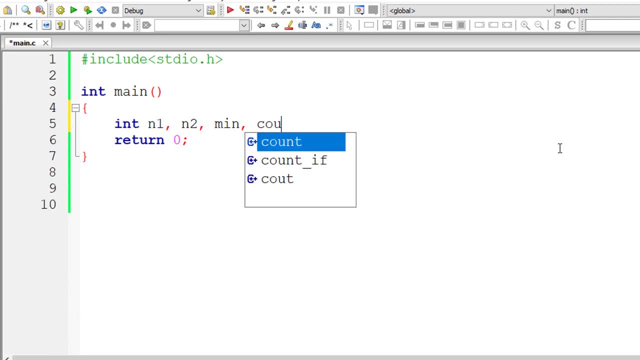 take integer variables n1 and n2 and min variable and a loop counter and flag. We assign 1 to flag, assuming user entered number or co-prime numbers. So I'll ask the user to enter two positive numbers and store it inside the address of integer variables n1 and n2.. Now I'll calculate. 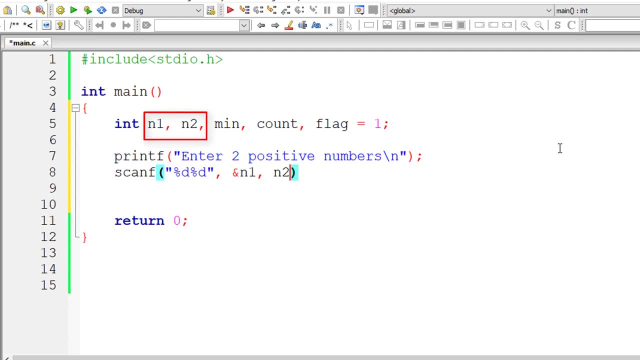 the smallest of two numbers, that is n1 and n2, and store it inside the variable min. So let me use ternary operand. So I'll take integer variables n1 and n2 and store it inside the operator. So min is equal to n1 if n1 is less than. 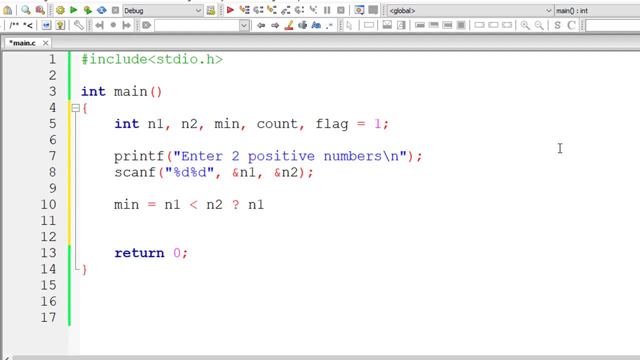 n2.. In that case, return the value of n1. if not, return the value of n2.. That's it. So let's write for loop I'll. I'll initialize count loop counter to two, because all the numbers are divisible by 1.. So we'll skip 1 and start with 2.. So loop executes iterates. 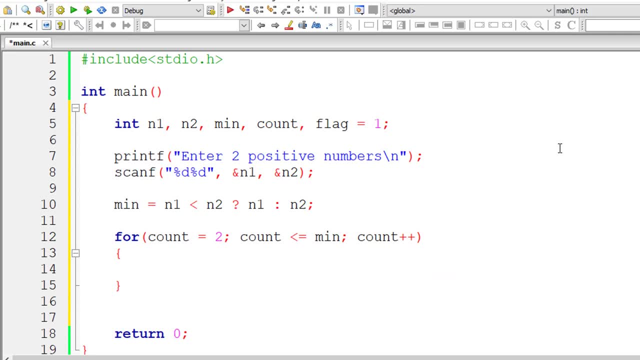 until count value is less than or equal to min. So this count value increments by 1 for of this for loop, inside for loop, i'll check if n1 modulo division count is equal to zero as well as n2 modulo division count is equal to zero. so both the user entered number should be perfectly. 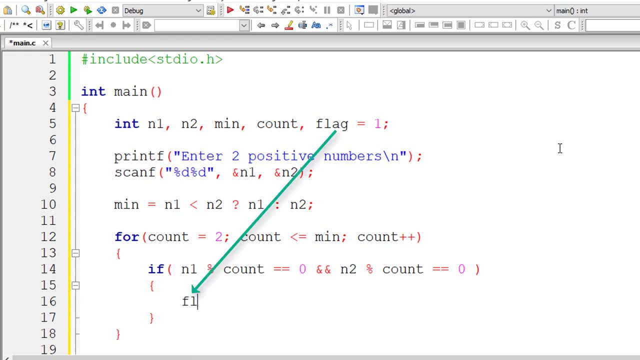 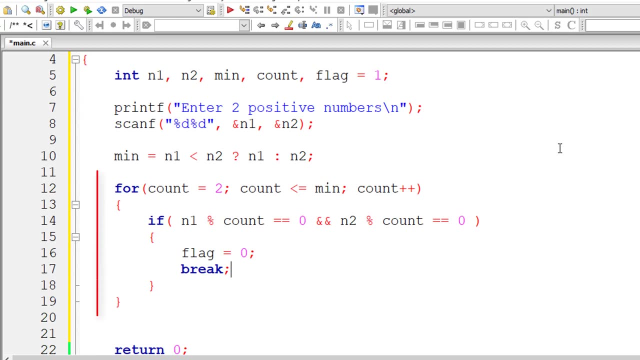 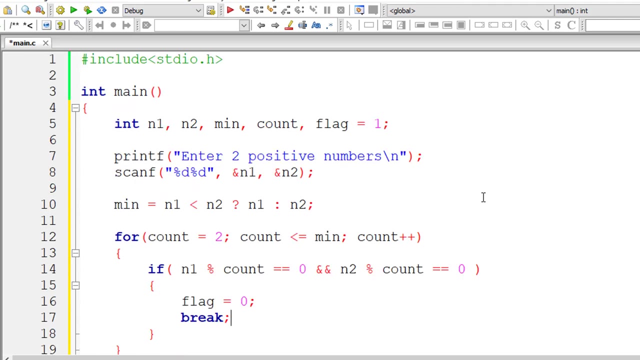 divisible by the value of count. in that case this is not a co-prime number, so i'll assign zero to flag and break out of this loop. so some other number is perfectly dividing. our user entered number n1 and n2, both these numbers, so this is not co-prime number. okay, no other numbers. 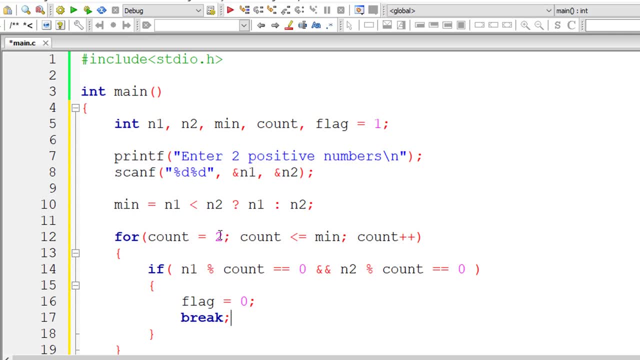 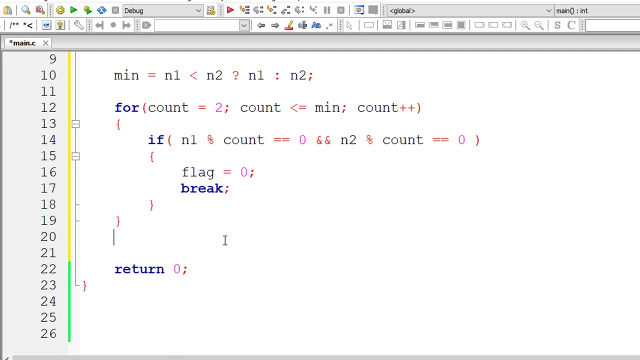 except one should divide both these numbers perfectly. that is, greatest common divisors for both these number, n1 and n2, should be 1.. if any other number that is common factor, common number, is dividing n1 and n2 perfectly, then this is not a these. these numbers are not co prime number. so 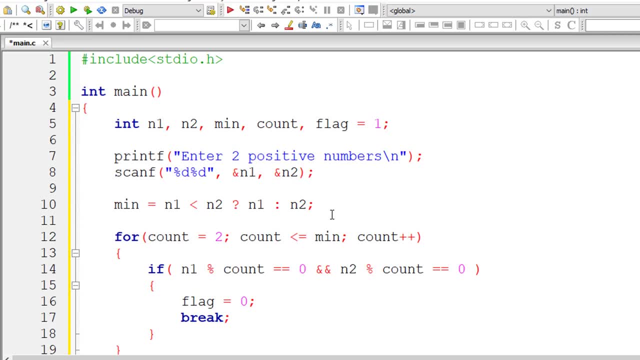 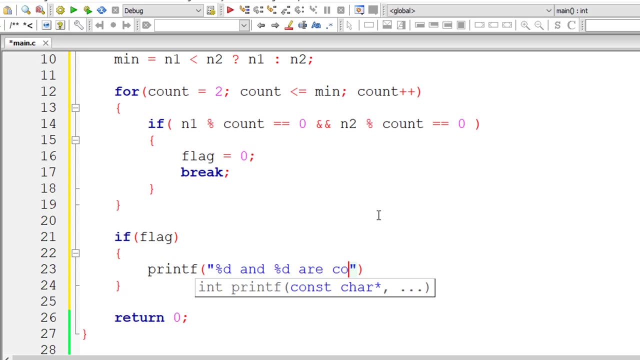 it if flag. in that case, if, after execution of this for loop, if flag value is still one, then these two numbers entered by the user are co-prime numbers. so percentage d and percentage d are co-prime. so the value is present inside variables n 1 and n 2. else that means if flag value is not.